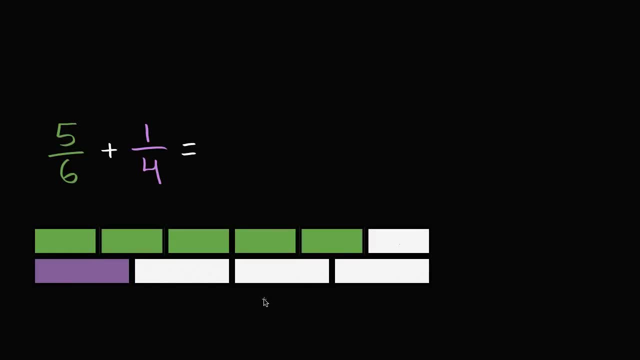 So this is 1- fourth And I want to add them, And I encourage you at any point, pause the video and see if you can figure it out on your own. Well, whenever we're adding fractions, we like to think in terms of fractions. 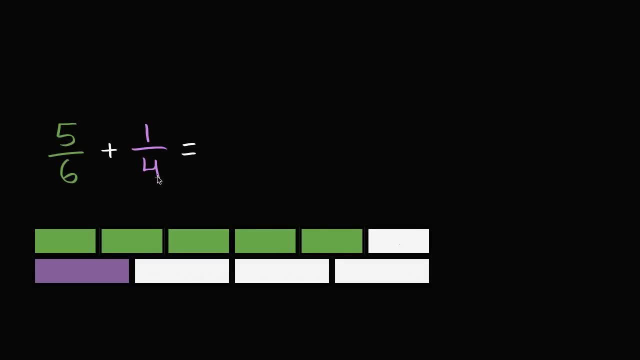 that have the same denominator And these clearly don't have the same denominator. But in order to rewrite them with a common denominator, we just have to think of a common multiple of 6 and 4, and, ideally, the smallest common multiple of 6 and 4.. 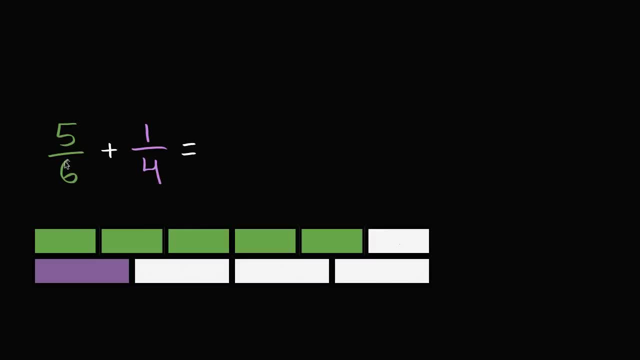 And the way that I like to do that is I like to take the larger of the two, which is 6, and then think about its multiples. So I could first think about 6 itself. 6 is clearly divisible by 6,, but it's not. 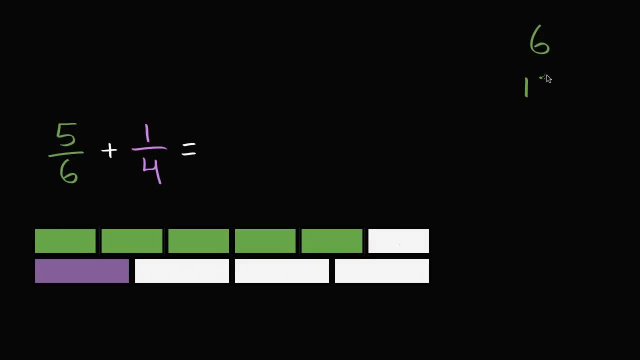 perfectly divisible by 4.. So now let's multiply by 2.. So then we get to 12.. 12 is divisible by both 6 and 4.. So 12 is a good common denominator here. It's the least common multiple of 6 and 4.. 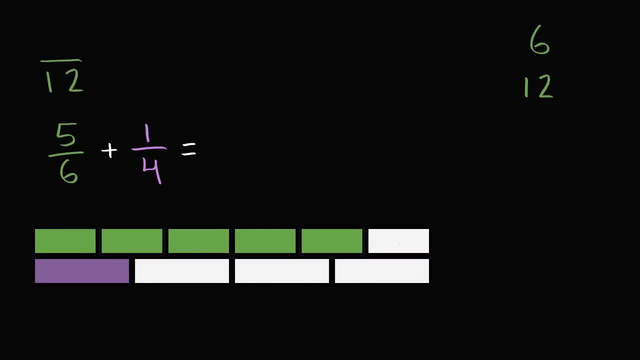 So we can rewrite both of these fractions as something over 12.. So something over 12 plus something plus 6.. Something over 12 is equal to Now. there's a bunch of ways to tackle it, but what I want to do is I just want to visualize it here. on this drawing. So if I were to go from 6 equal sections to 12 equal sections, which is what I'm doing, if I'm going from 6 in the denominator to 12 in the denominator, I'm essentially multiplying each of these sections by 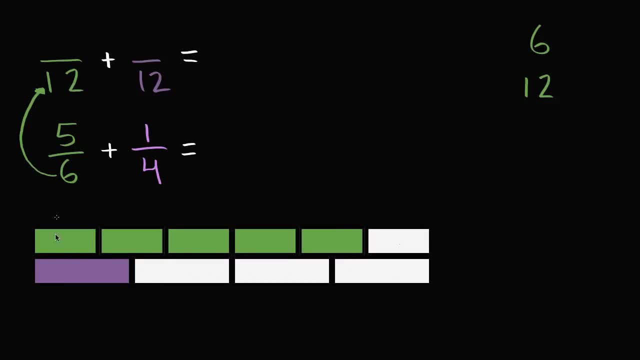 or I'm essentially multiplying the number of sections I have by 2, or I'm taking each of these existing sections and I'm turning them into two sections. So let's do that, Let's do that. Let me see if I can do it pretty neatly. 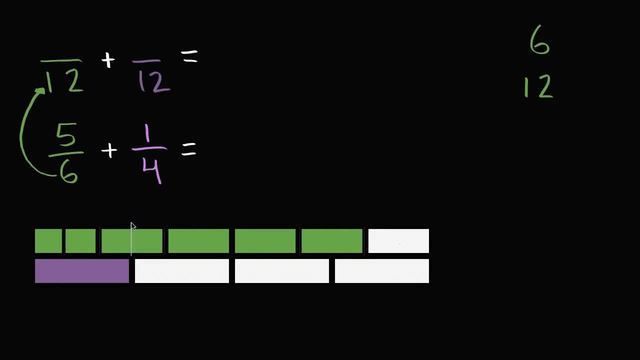 So I could do it a little bit neater than that. So it'll look like that: And whoops, Let me do this one. I want to divide them fairly close to evenly. I'm doing it by i, so it's not going to be perfect. 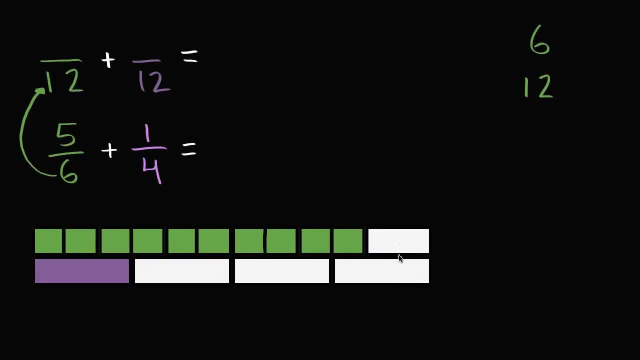 So then you have that one, and then, last but not least, you have that one there, And then notice, I had 6 sections, but now I've doubled the number of sections. I've turned the 6 sections into 12 sections. 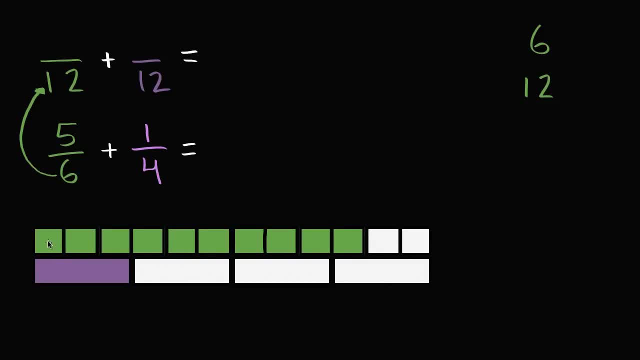 by turning each of the original 6 into 2.. So now I have 1,, 2,, 3,, 4,, 5,, 6,, 7,, 8,, 9,, 10,, 11,, 12 sections. 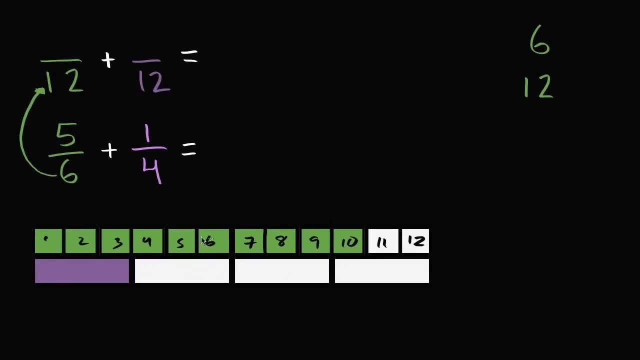 So if I have 12 sections, I'm going to multiply each of these sections. So if I have 12 sections, now how many of those 12 are now shaded in? Instead of having 5 of the 6,, I now have 10 of the 12 that are shaded in. 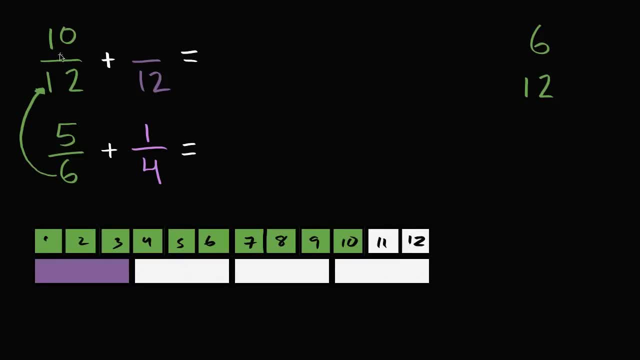 So I now have 10 twelfths. 5, 6 is the same thing as 10 twelfths. Another way you could have thought about that: to go from 6 to 12, I had to multiply by 2.. 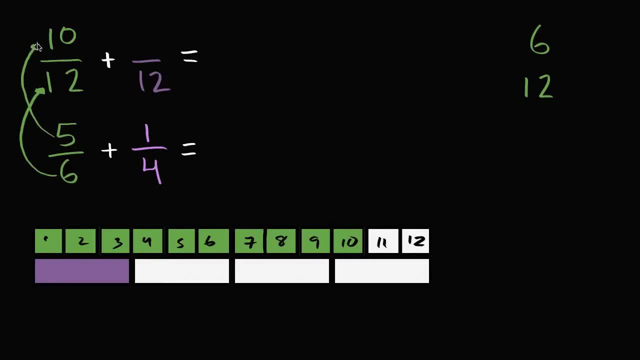 So then I have to do the same thing in the numerator. 5 times 2 is 10.. But hopefully you see that those two fractions are equivalent, that I didn't change how much is shaded in. I just took each of the original 6 and I turned it into 2,. 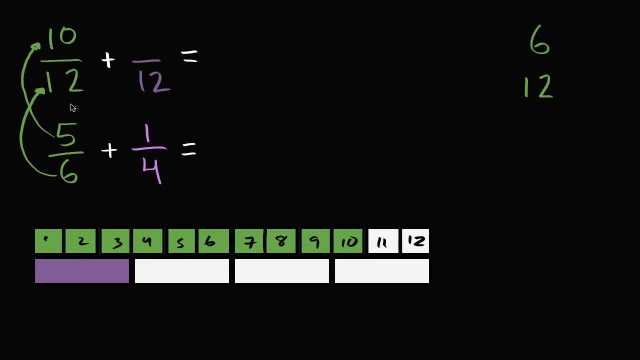 or I multiplied the total number of sections by 2 to get 12.. And then, instead of having 5,, 6,, I now have 10 twelfths shaded in. Now let's do the same thing with the 4,, with the 1 fourth. 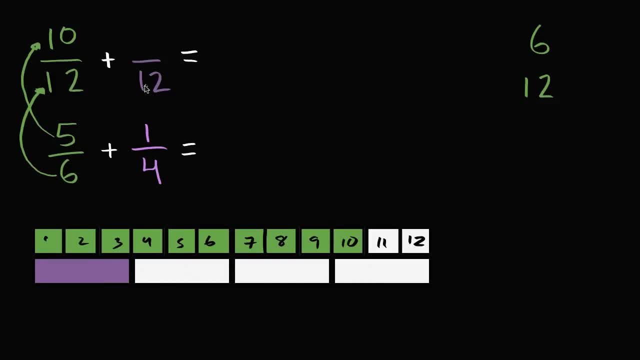 Right here I've depicted 1- fourth, but I want to turn this into something over 12.. So to turn it over something over 12, each section has to be turned into 3 sections. So let's do that. Let's turn each section into 3 sections. 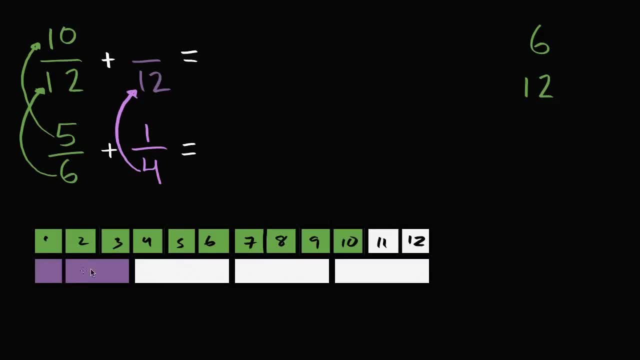 So let's do that. Let's turn each section into 3 sections, So that's 1,, 2, and 3.. So then I have 1,, 2, and 3.. I have I think you see where this is going. 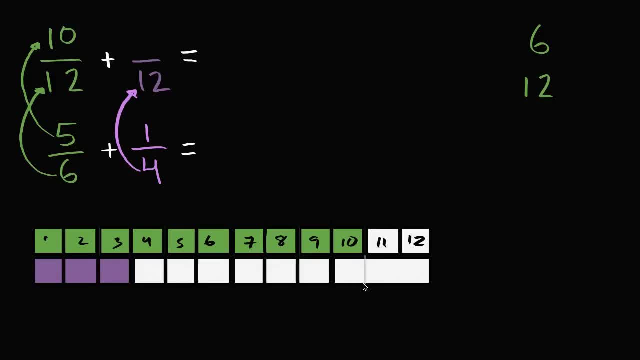 1,, 2, and 3.. I have 1,, 2, and 3. And so, notice, all I did is I multiplied. before I had 4 equal sections. now I turned each of those 4 sections into 3 sections. 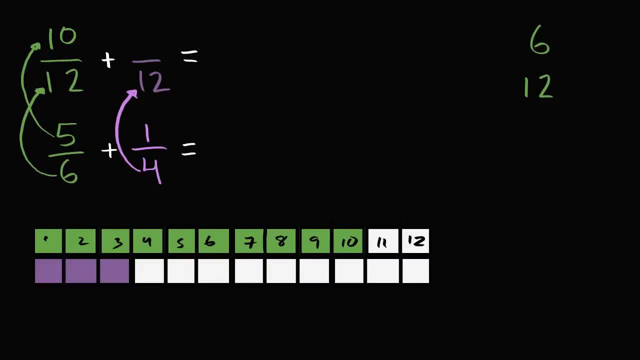 So now I have 12 equal sections, And I did that essentially by multiplying the number of sections I had by 3.. So now, what fraction is shaded in? Well, now, this original that was 1 out of the 4, we can now see is 3 out of the 12 equal sections.